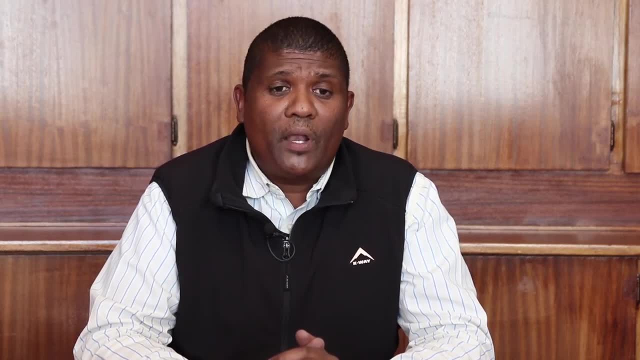 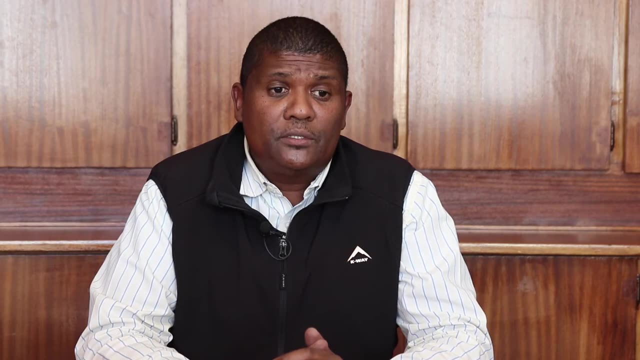 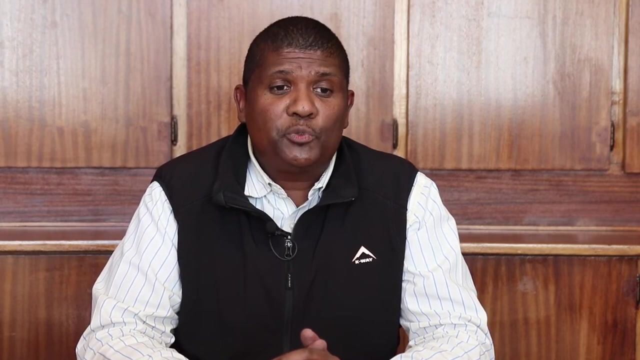 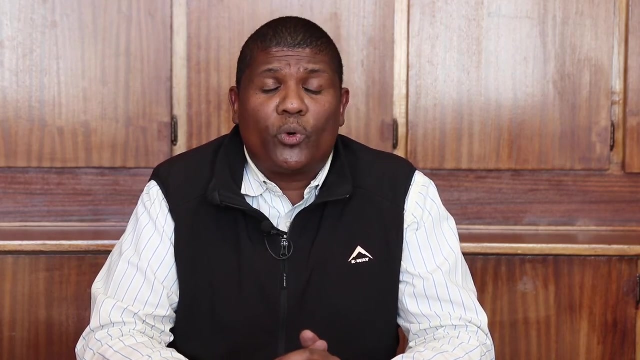 soil issues further to understand the complexities of soil sampling and analysis. OMBO introduction to GIS will give the student basic theoretical background in GIS and some practical experience in GIS analysis and map design. OMBO 6-1-4- GIS Applications was designed to build on the introductory 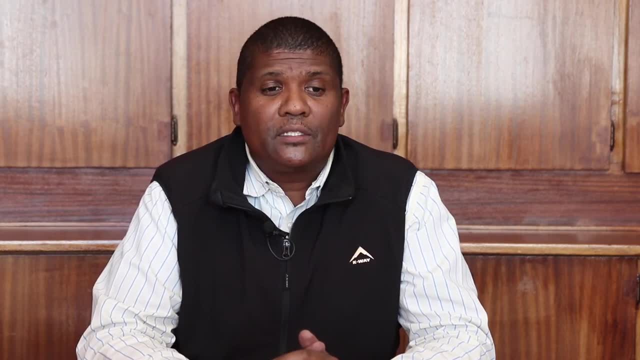 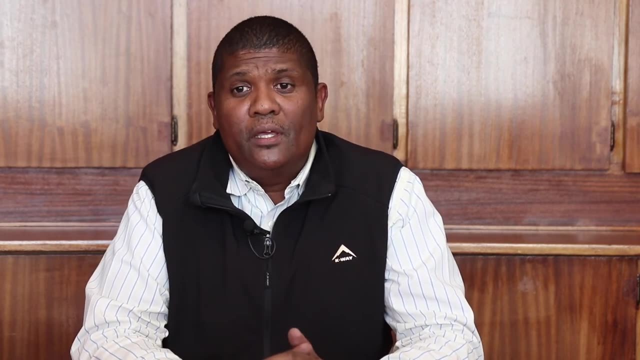 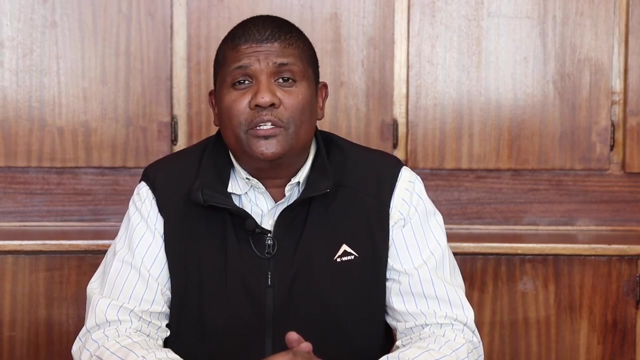 GIS module and focus on data analysis and spatial modeling. in environmental sciences. OMSB 6-1-1- Conservation Ecology integrates the academic domains of ecology and conservation biology. there is a emphasis on Silicon Valley analysis. OMSB disciples focus on the H clique- landscapes. 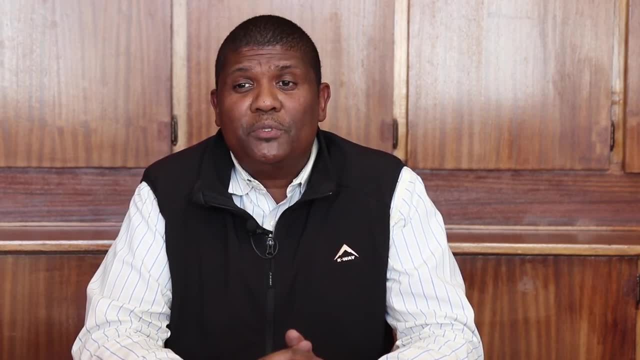 VR deles he這種 committees y program bareijaring rob action plan学cessiva animat beter id presets מס denominat bachelor ouvence st LOVE products, omsba. ze shift from control or management of species and habitat to facilitating evolutionary processes. 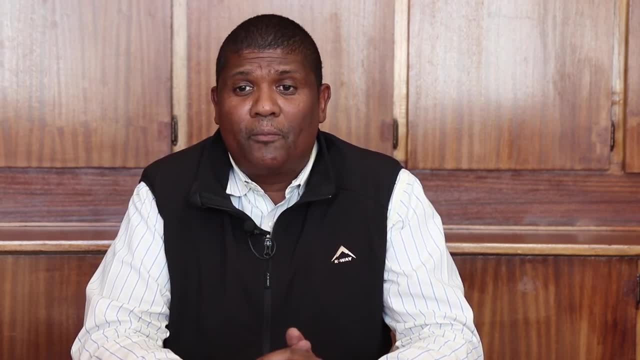 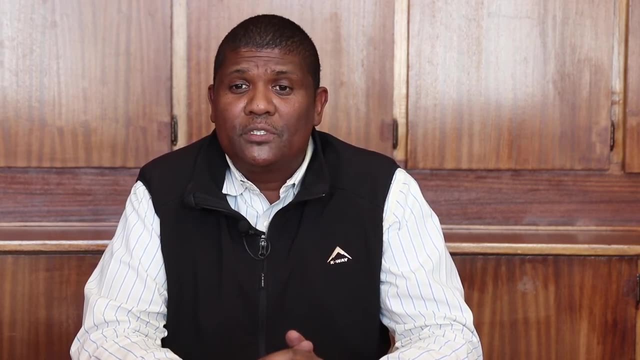 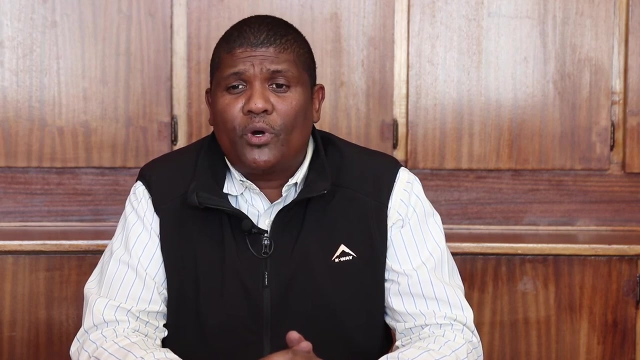 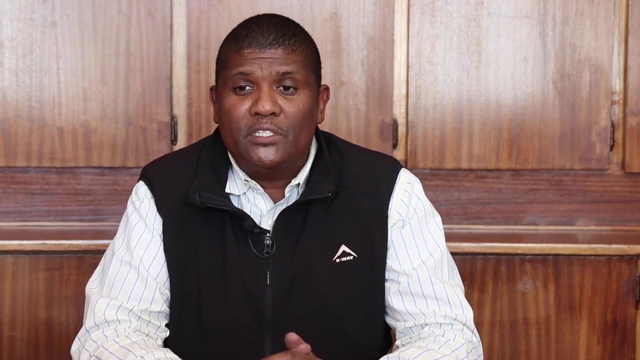 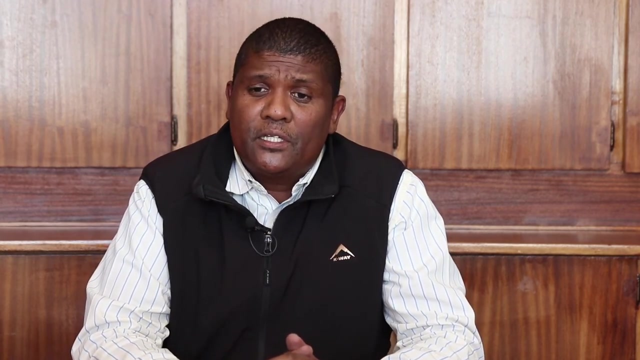 and anthropogenic change with decision making. OMSE 621- Restoration of Degraded Ecosystems is focused on the long-term sustainability of rangeland management strategies. further to understand the complex nature of community-based natural resource management principles in rangeland management and restoration ecology- OMSE 622- Urban Ecology is an introductory course. 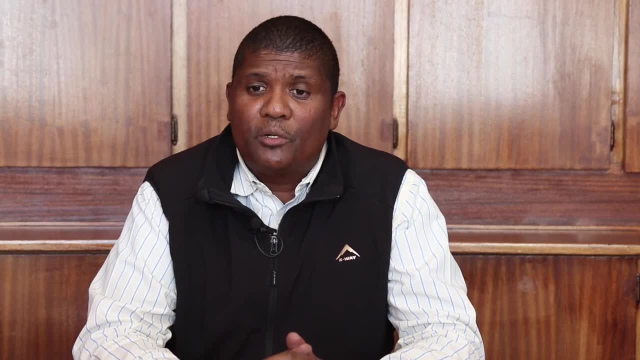 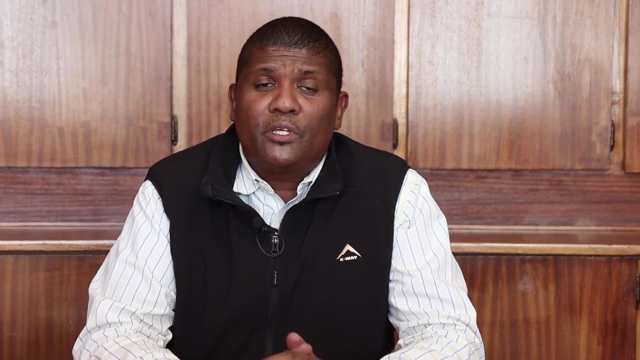 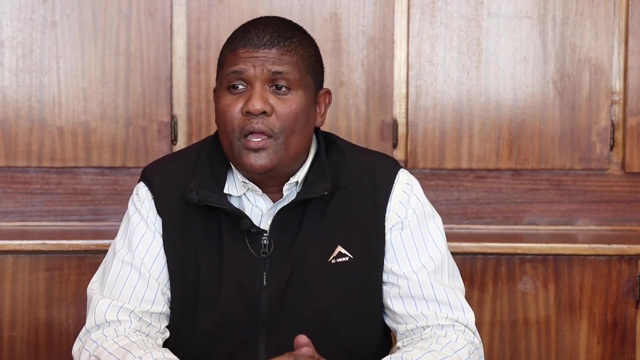 in which the scope and historical development of urban ecology, different approaches in urban ecological studies and the application of urban ecological principles are covered. OMSE 623- Plant Ecophysiology and Stress. Physiology focuses on the physiological and biochemical responses of plants to environmental stress. The module also covers 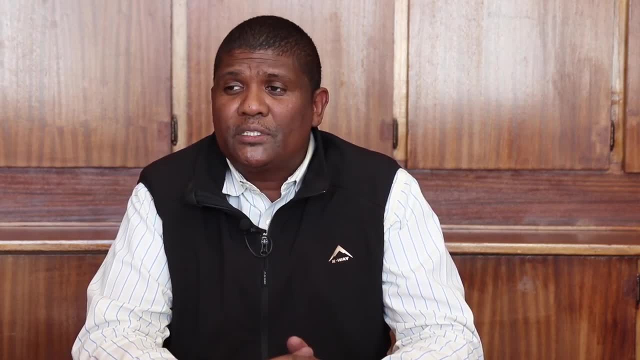 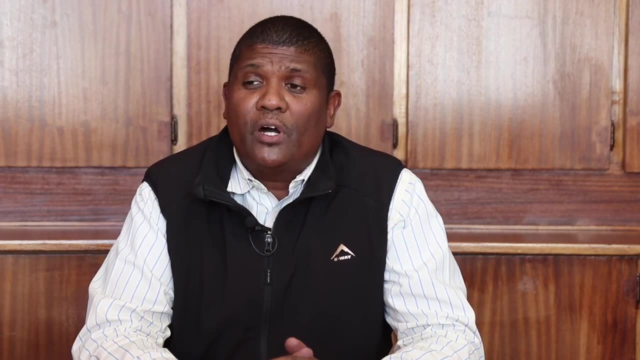 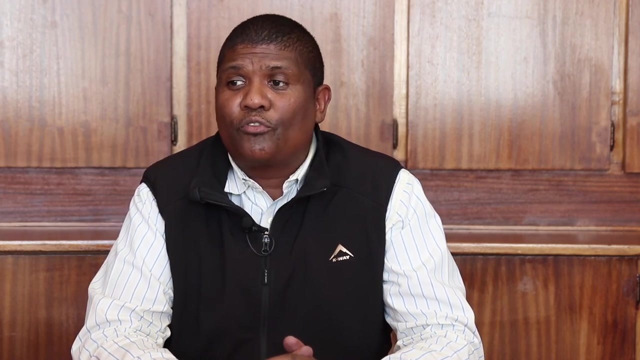 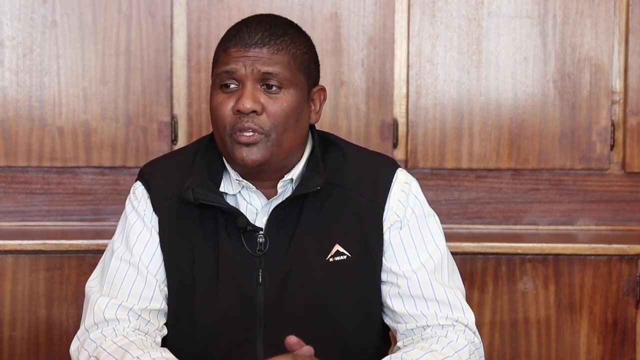 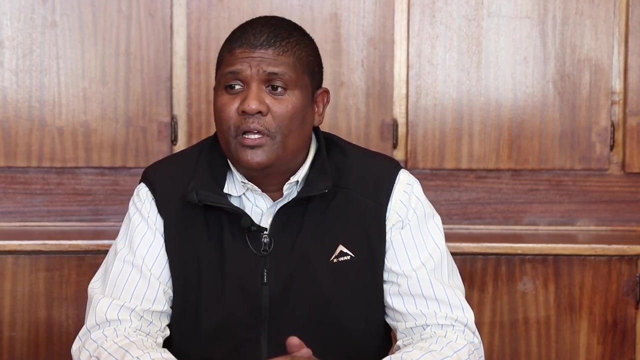 the physiological acclimation and adaptation strategies of plants to changes in their environment. OMSE 625- Advanced Ecotoxicology focuses on understanding the effects of contaminants on organisms in the environmental. This module will give students insights on the application of toxicity testing using standard test methods in the field of environmental risk assessment.